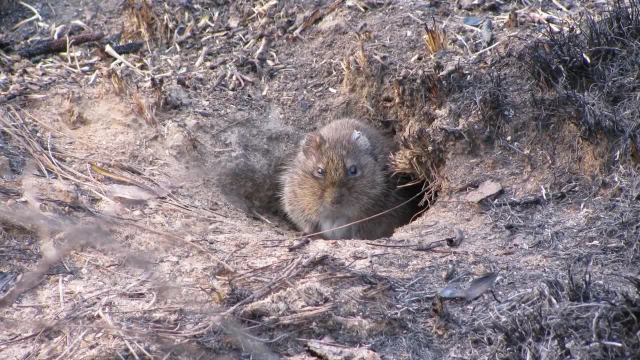 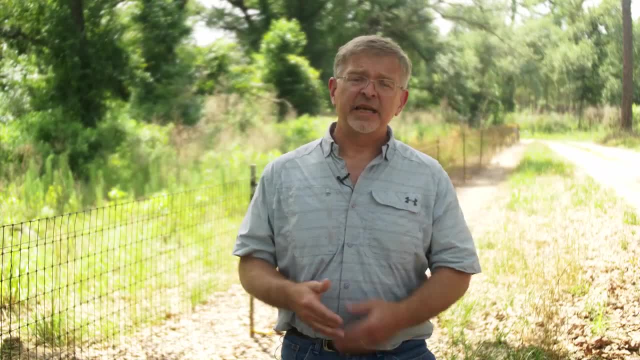 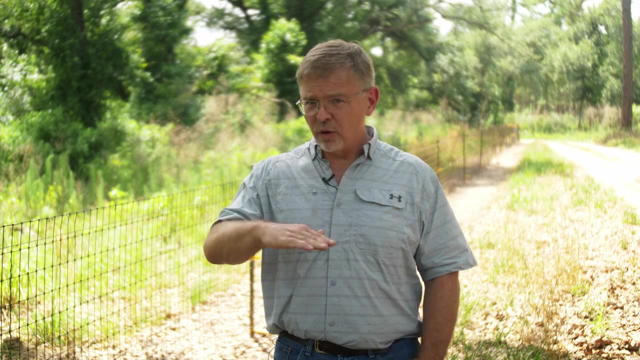 And one of them in particular, which is the hispid cotton rat. if it's not the most common, it's tied for the most common small mammal on the property. That species makes up probably- I think it's safe to say- 50 percent of the diet of most of our predator species here. 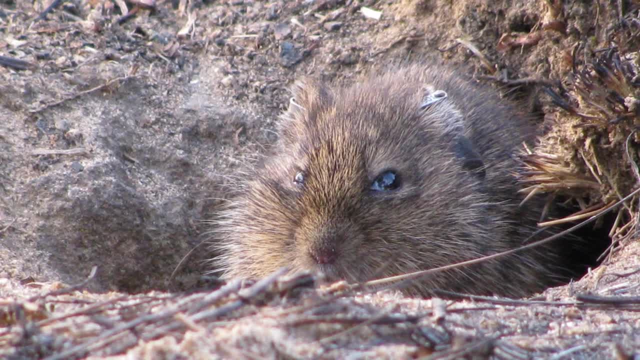 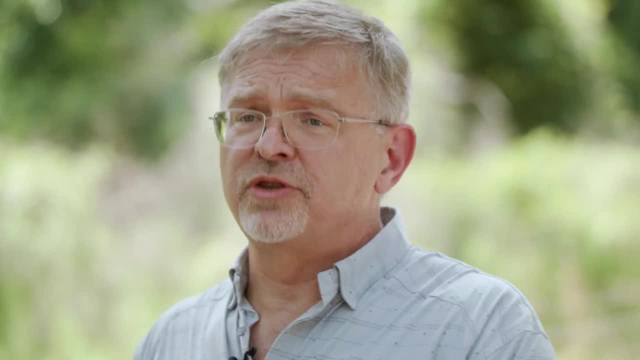 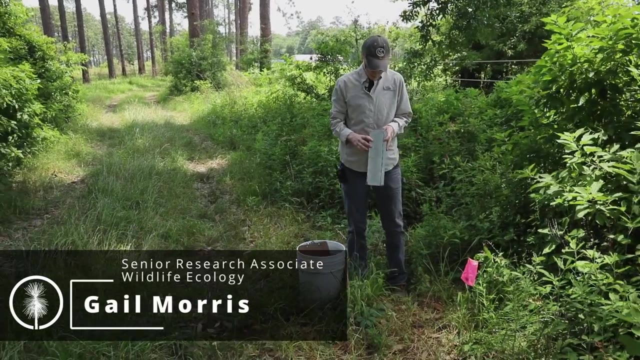 So they're that important And so it's important that we know where these animals are, how our management, especially prescribed fire, affects their populations, because they're the species that hold up the predator community. We are small mammal trapping. We set a bunch of these Sherman live traps out and 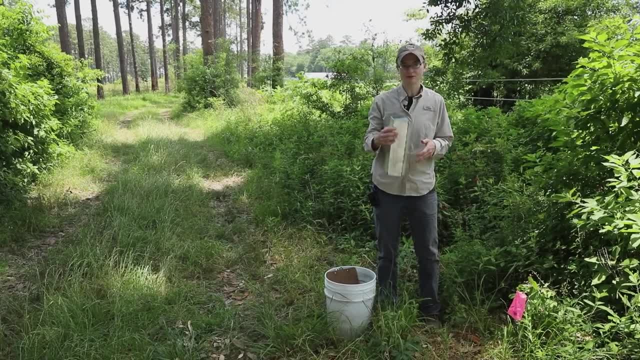 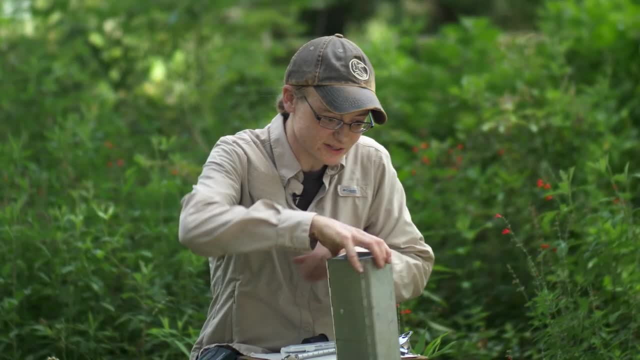 put some bait in it and left them overnight And we caught a hispid cotton rat here And now. we're going to take some biological data from this rat. So this animal does not have any your tags, which means we've never caught it before. So one of the things we typically 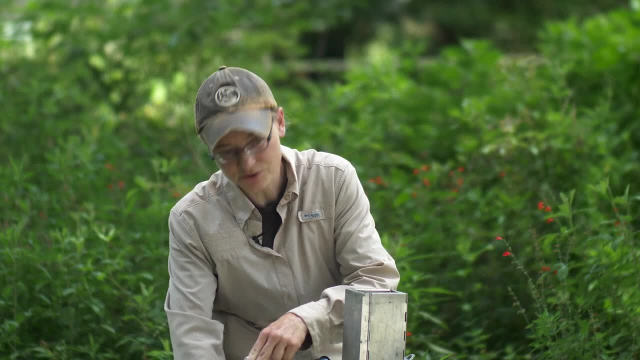 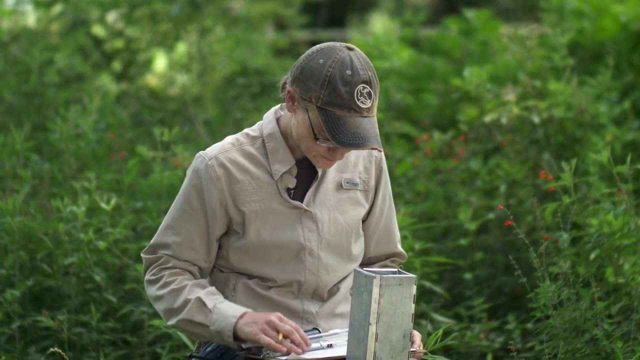 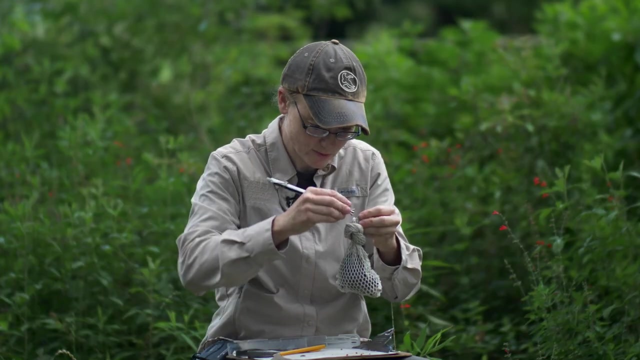 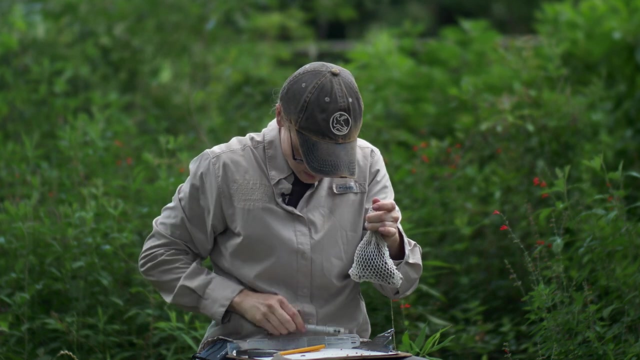 do is we will put in your tag on these animals so that in the future, if we recapture them, we will have that information to know that this is an animal that we've had before And you can do a lot of data analysis with that kind of mark: recapture data. She weighs 132 grams. That's. 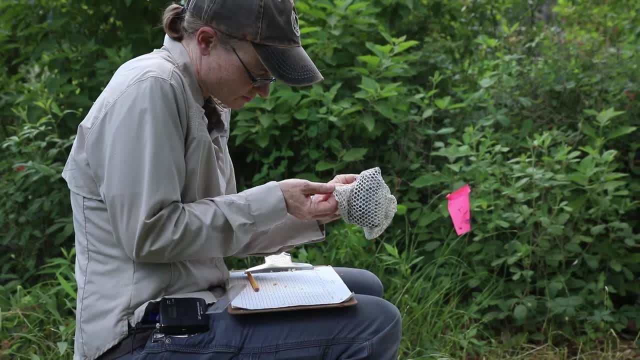 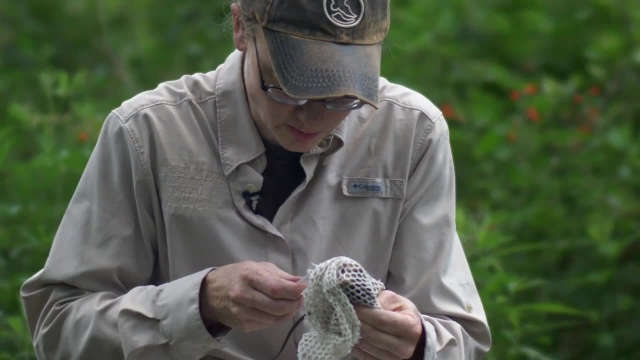 actually a pretty good fish And she weighs, I'm guessing, about 78 grams, So that's a pretty good, a pretty good sized rat. So one of the things we take is the hind foot length, which we just measure the longest toe on one of the feet. 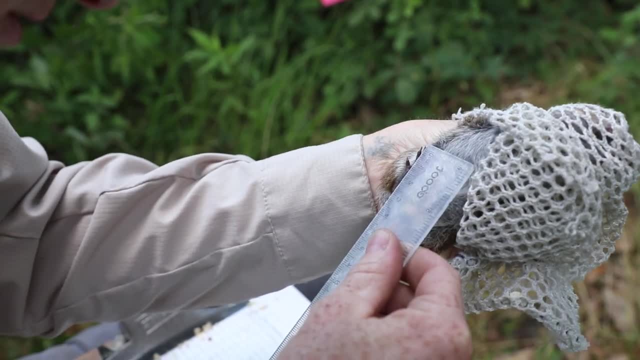 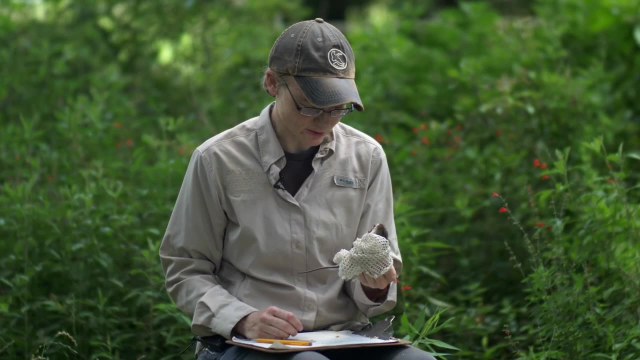 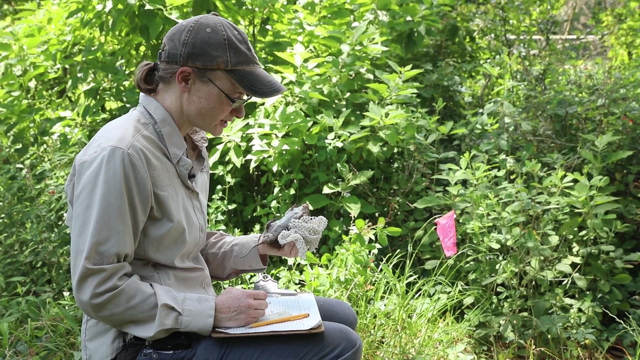 And her hind foot is about 27 millimeters. I think they just play a really interesting ecological role in this ecosystem. A number of years ago we did a research project where we put radio- tiny little radio collars on these guys and we tracked them and were interested in what. 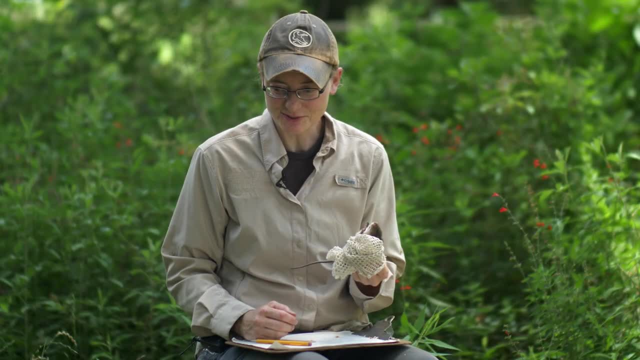 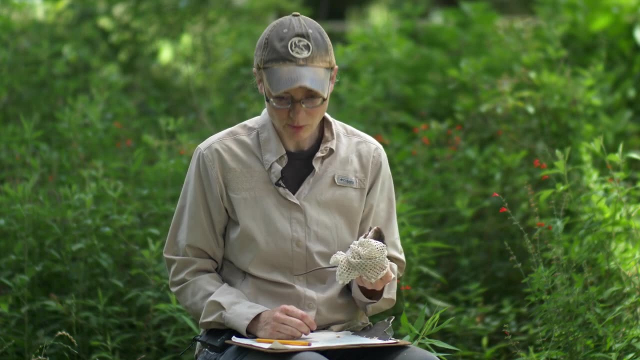 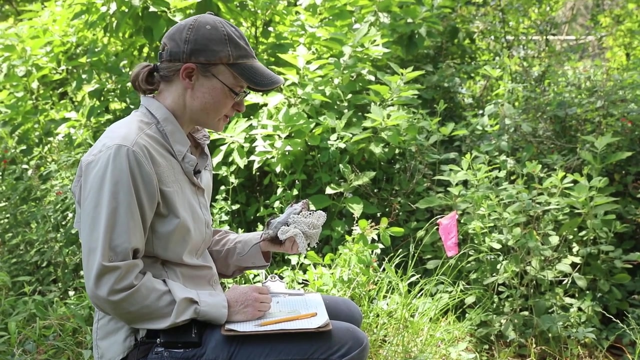 the cause of death was for them And basically what they do is they sort of like feed everything up the food chain. We found them in five different species of snakes. We found them in owl pellets, in hawks nests, We found them in raccoon poop and bobcat poop and coyote poop, And so I find that by.